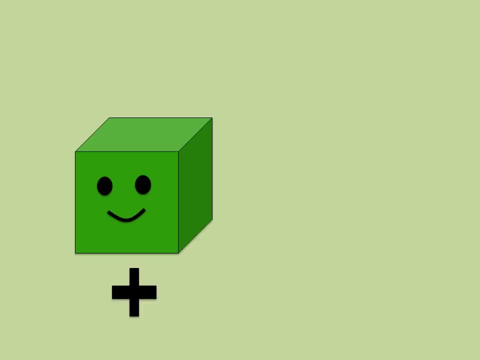 is happy and has a very positive attitude. Let's use this red block to represent negative. This block is grumpy and full of negativity. Do you want to share some pie with me? No, I hate pie and I'm probably allergic. So now we have a way of representing both positive. 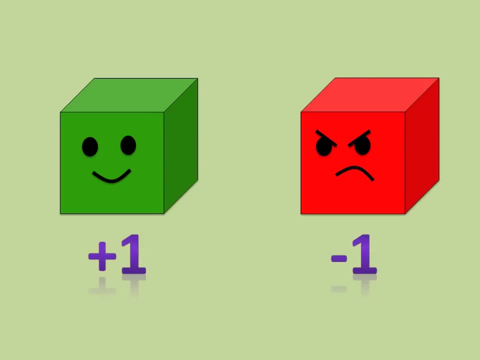 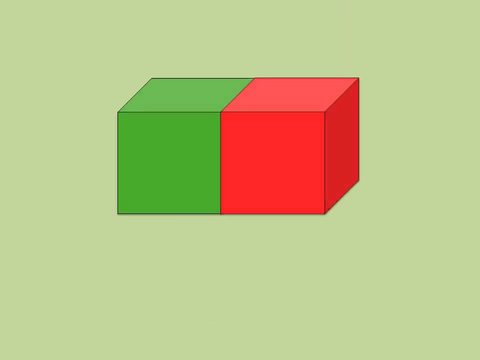 numbers and negative numbers. What do you think will happen if we put them together? Well, I think we're about to find out. Well, isn't that something? There's exactly as much positive as there was negative, and they just burned each other out. What this shows. 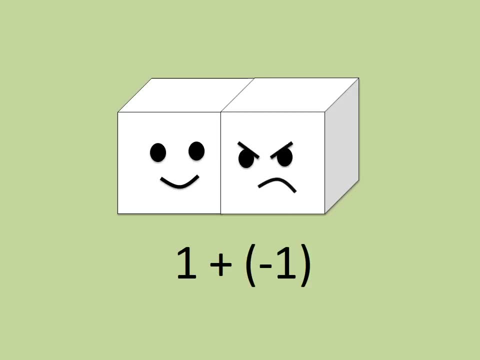 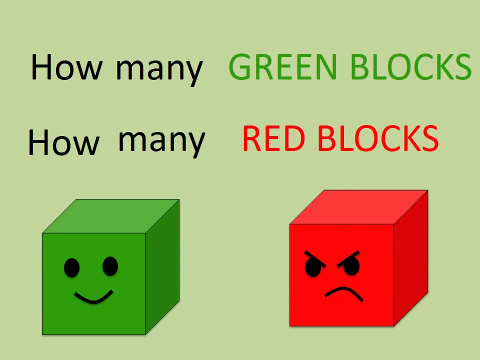 to us is positive one and negative one equals zero. Our plan for the next few problems will be to figure out how many green blocks and how many red blocks you'll need. The formula is based on the size of the numbers and the sign in front of them. Let's try. 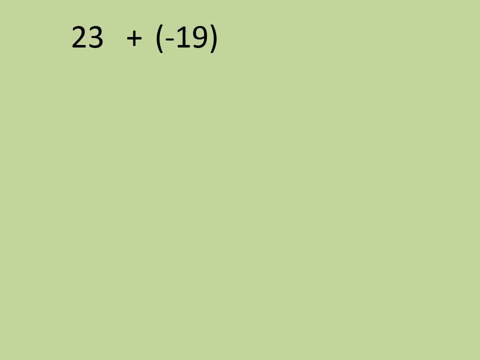 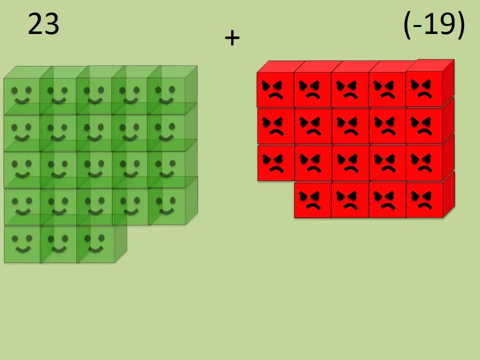 23 plus negative 19.. Let's move these over here so we can have as much space as possible. So remember we're going to use green blocks to represent positives and red blocks to represent negatives. So we have 23 green blocks and 19 red blocks. 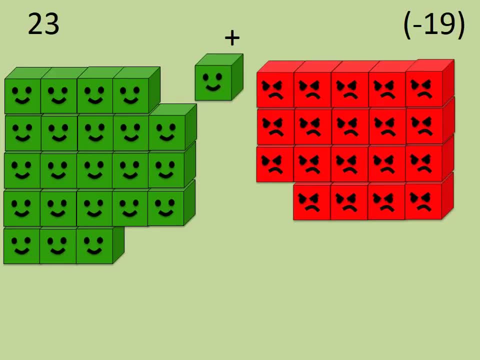 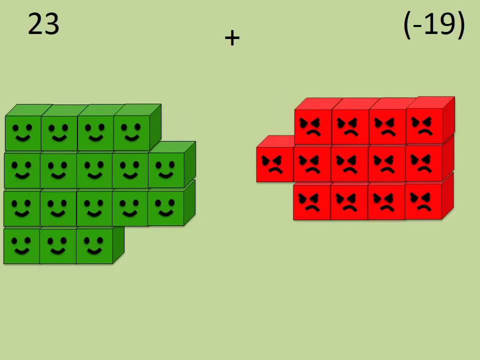 So remember, when one of these positive green blocks meets one of these negative red blocks, they equal zero. They go away. Let's do the same thing for all of these. There we go. Yep, Let's get rid of that one and this one, and this one and this one. 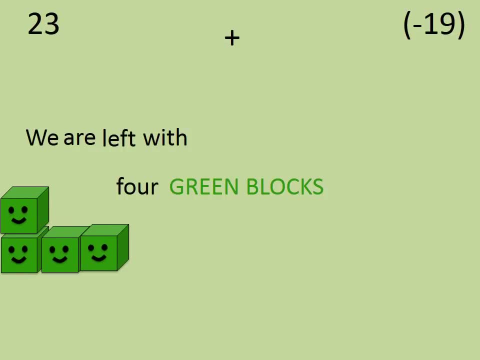 All right, We are left with four green blocks. What does that mean? Well, remember, the green blocks were positive, so we have positive four. So 23 plus negative 19 is positive four. We did this by counting out 23 green blocks and 19 red blocks. 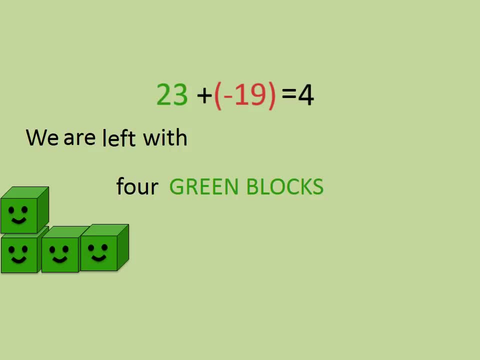 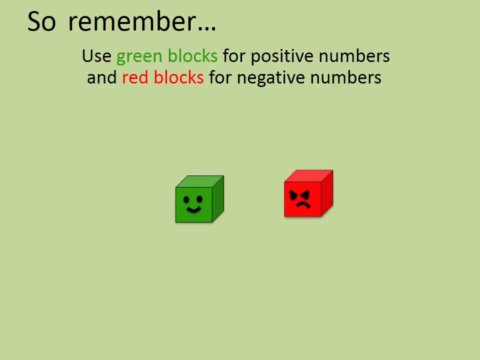 Then we paired them together until we ran out of one color block and counted how many of the other color we had left Neat. So remember, use the green blocks for positive numbers and red blocks for negative. Make and remove the red-green block pairs like this: